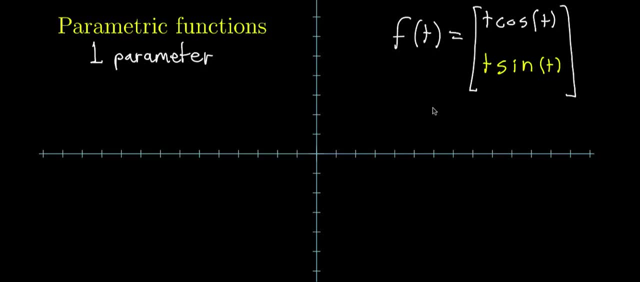 so I'll go ahead and draw a coordinate plane here And let's just evaluate this function at a couple different points and see what it looks like. okay, So I might. maybe the easiest place to evaluate it would be zero. So f of zero. 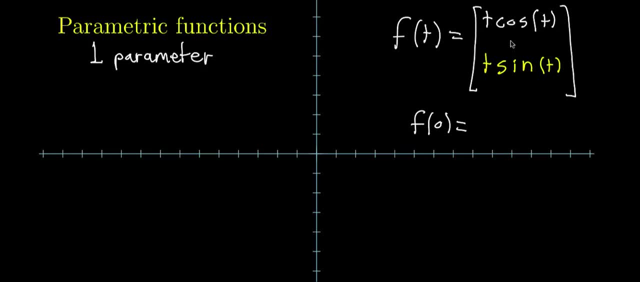 is equal to, and then in both cases it'll be zero times something. so zero times cosine of zero is just zero, and then zero times sine of zero is also just zero, So that input corresponds to the output. You could think of it as a vector that's infinitely small. 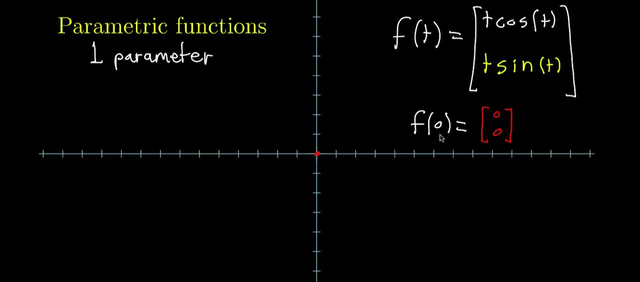 or just the point at the origin, however you want to go about it. So let's take a different point, just to see what else could happen. And I'm going to choose pi halves, Of course. the reason I'm choosing pi halves: 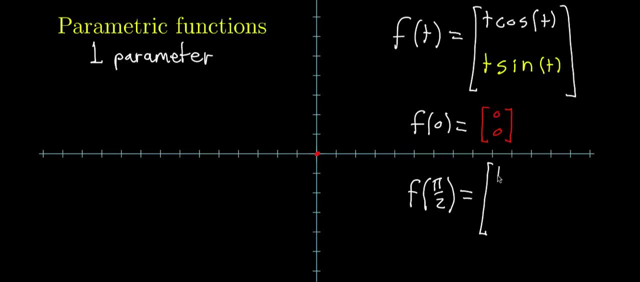 of all numbers is that- it's something I know how to take- the sine and the cosine of So t is pi halves, cosine of pi halves. And you start thinking, okay, what's the cosine of pi halves, What's the sine of pi halves. 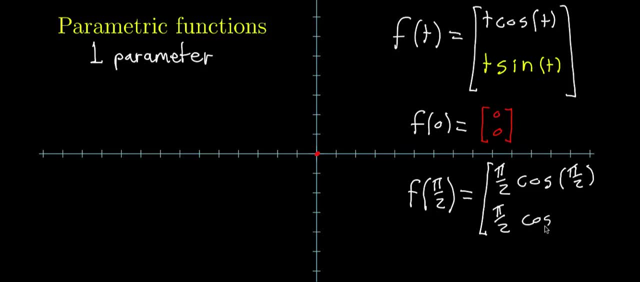 And maybe you go off and draw a little unit circle while you're writing things out. Oops, This is the problem with talking while writing Sine of pi halves, And you know it's if you go off and scribble that little unit circle. 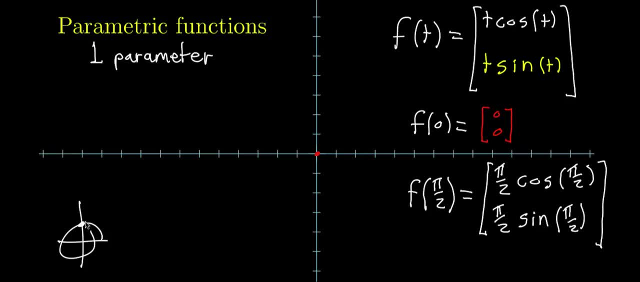 and you say pi halves is going to bring us a quarter of the way around over here, and cosine of pi halves is measuring the x component of that, so that just cancels out to zero. And then sine of pi halves is the y component of that. 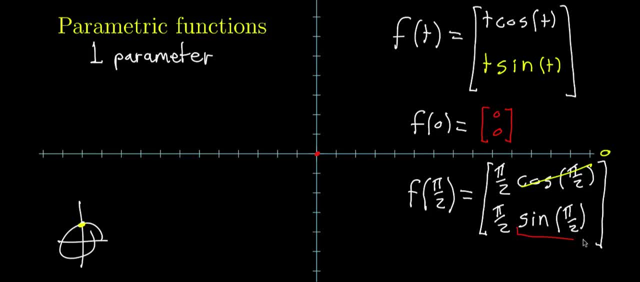 so that ends up equaling one, which means that there's something in there that's equaling two. The vector as a whole is gonna be zero for the x component and then pi halves for the y component, And what that would look like. 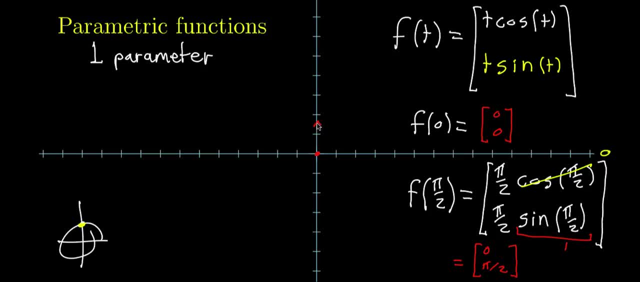 you know, the y component of pi halves- it's about 1.7 up there- and there's no x component. so you might get a vector like this And if you imagine doing this at all the different input points, you might get a bunch of different vectors. 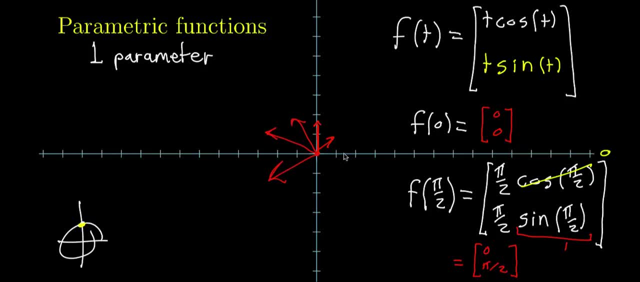 off doing different things. And if you were to draw it, you don't wanna just draw the arrows themselves, because that'll clutter things up a whole bunch. So we just wanna trace the points that correspond to the output, the tips of each vector. 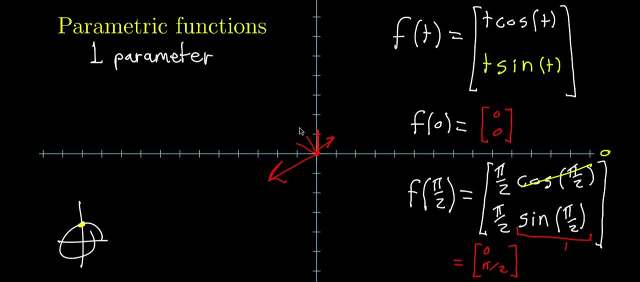 And what I'll do here. I'll show a little animation- Let me just clear the board a bit- An animation where I'll let t range between zero and 10. So let's write that down. So the value t is gonna start at zero. 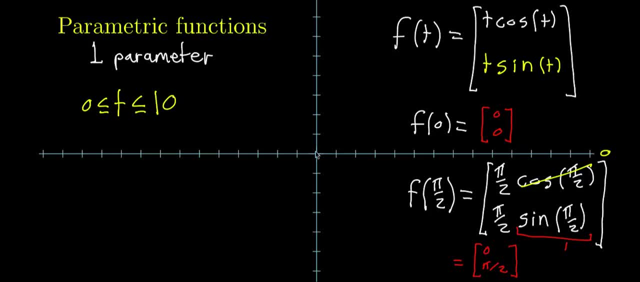 and then it's go to 10,, it's gonna go to 10. And we'll just see what values, what vectors does that output And what curve does the tip of that vector trace out? So here it goes, all of the values. 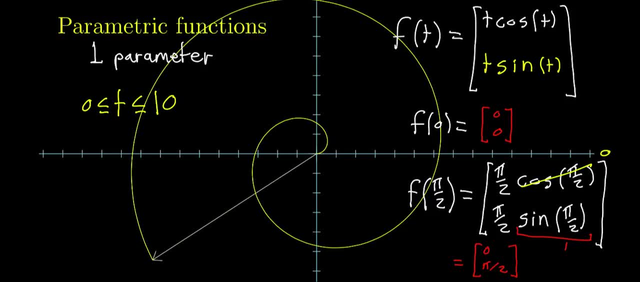 just kind of ranging zero to 10. And you end up getting this spiral shape And you can maybe think about why this cosine of t, sine of t, scaled by the value t itself, would give you this spiral. But what it means is that when you 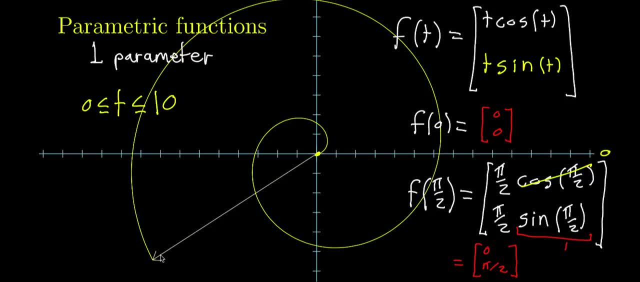 you know, we saw that zero goes here. evidently It's the case that 10, and 10 outputs here, And a disadvantage of drawing things like this. you're not quite sure of what the, what, the interim values are. You know, you could kind of guess. 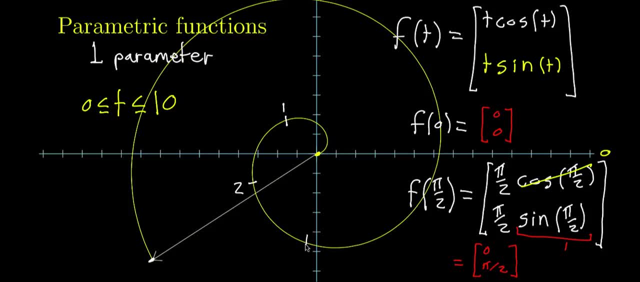 maybe one goes somewhere here, two go somewhere here And you're kind of hoping that they're evenly spaced as you move along. But you don't get that information. You lose the input information. You get the shape of the curve And if you just want you know. 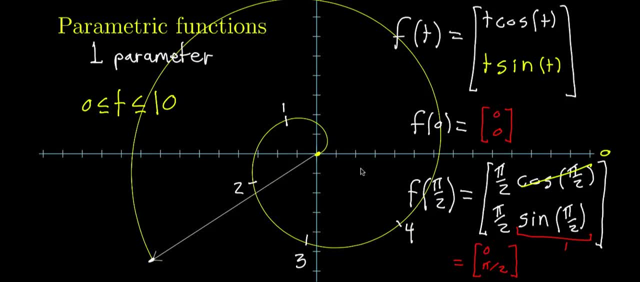 an analytical way of describing curves. you find some parametric function that does it And you don't really care about the rate. But just to show where it might matter, I'll animate the same thing again. Another function that draws the same curve. 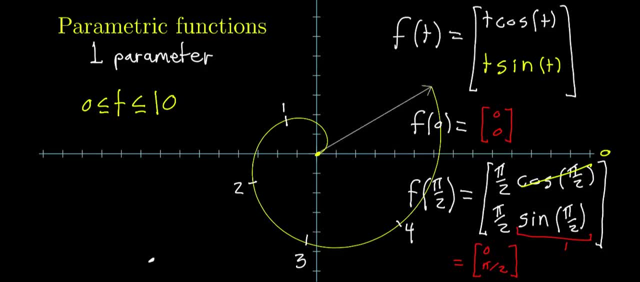 but it starts going really quickly And then it slows down as you go on. So that function is not quite the t cosine t, t sine of t that I originally had written, And in fact it would mean that let's just erase these guys. 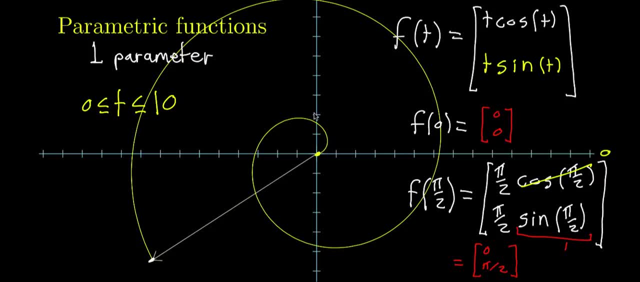 When it starts slowly, you can interpret that as saying, okay, maybe, well, actually it started quickly, didn't it? So one would be really far off here, And then two zipped along here And then three, you know, still going really fast. 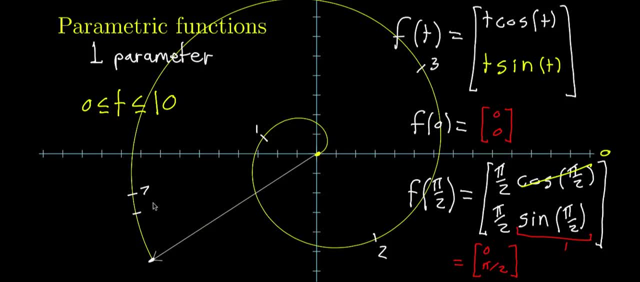 And then maybe by the time you get to the end, it's just going very slowly, just kind of: seven is here, eight is here and it's hardly making any progress before it gets to 10.. So you can have two different functions.